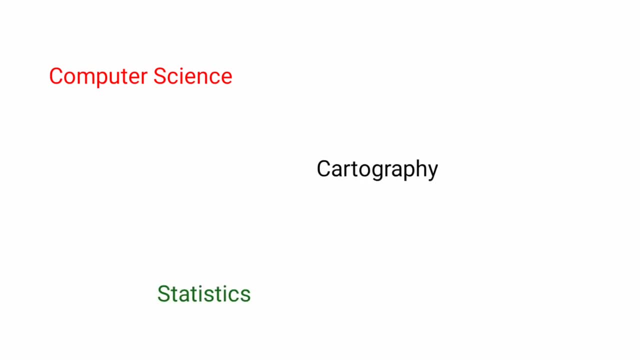 as computer science, statistics, cartography, remote sensing, database technology, geography, geology, hydrology, agriculture, resource management, environmental science and public administration. So what are the basic components that a GIS requires? So the important components of a geographical information system include hardware, software. 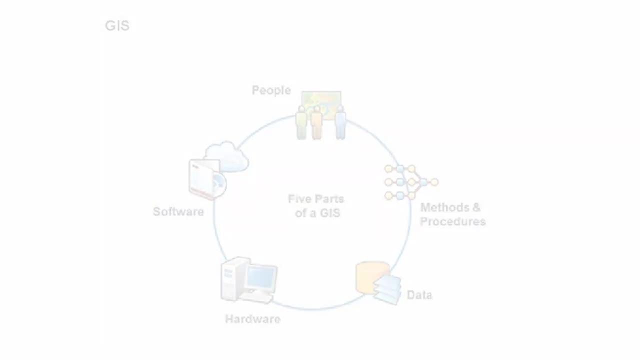 data, people and procedures. So the next question arises: how does a GIS work? So there, the sequence of the activities that are involved in GIS related work are as follows: In the first, the spatial data input, which refers to acquiring database from various 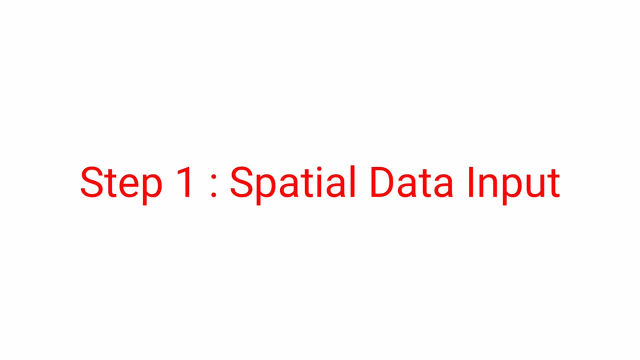 sources. Data is to be sorted out before it is entered, So the purpose and the aim of data, the maps, should be studied thoroughly. The second step involves entering of the attribute data. Now the data is selected, it needs to be entered on the GIS software. 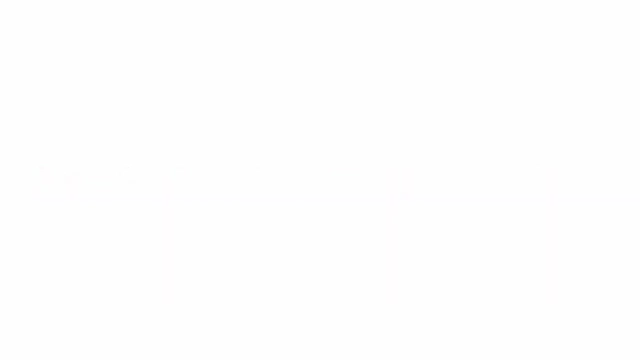 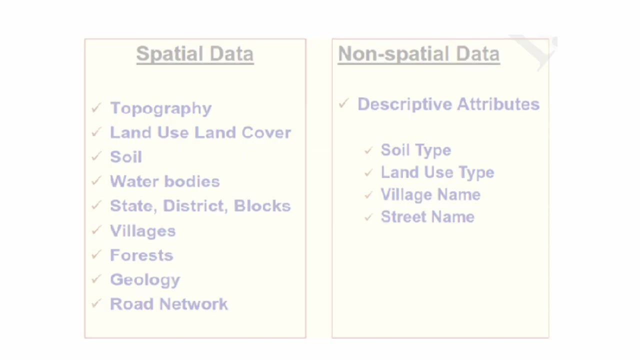 Lastly, the spatial data is entered and is followed by the non-spatial data or the attribute data. You can understand the difference between them by a single example On a Google map when you search for a place like, just for an instance, your school. so 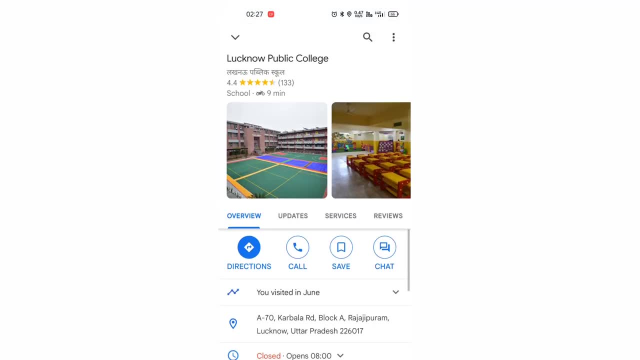 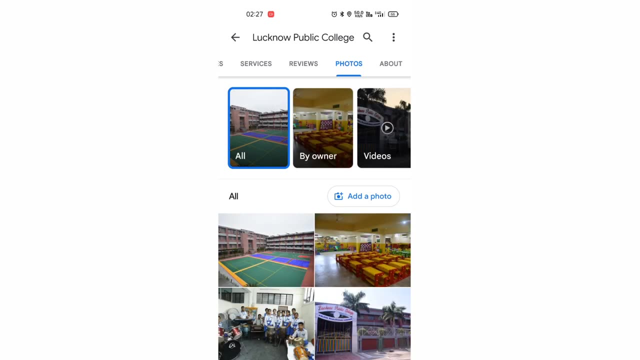 your school is the spatial data, While when you click on your school, you will find which board it is affiliated to or what facilities your school gives, which courses are provided, what sports facilities are available. So the properties are termed as a non-spatial data or the attribute data. 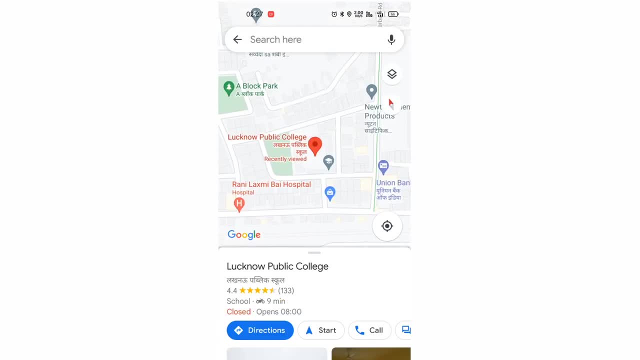 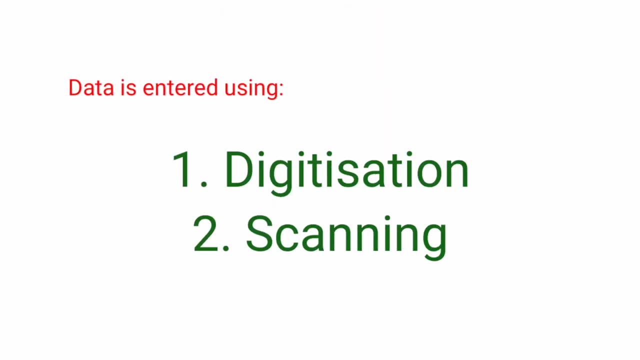 So this is the first step. The second step is to search for a place. The spatial data- The spatial data are the most important prerequisite in a spatial or geographical information system. Data is usually entered on a GIS software using two processes. The first is digitization and the second is scanning. 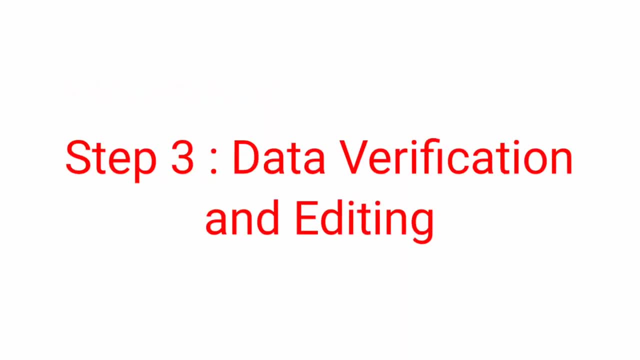 After the data is entered to the GIS software, the next step is data verification and editing, which implies the spatial data that is captured into a GIS software requires verification for the error identification and corrections so as to ensure the data accuracy. The errors caused during digitization may include data omissions and under end overshoots. 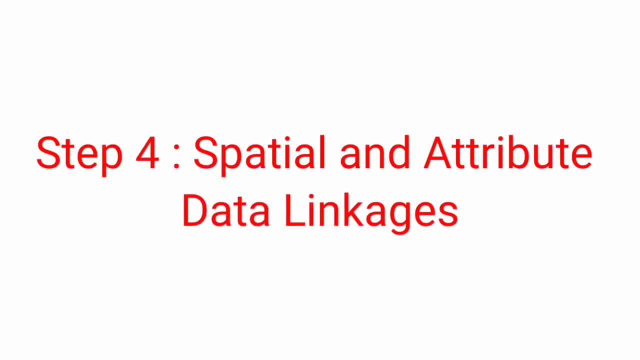 etc. After the data verification and editing, we move to the spatial and attribute data linkages, which means the process to link the spatial data to the non-spatial data And, lastly, the most important part, that is, spatial analysis. The strength of the GIS lies in its analytical capabilities.